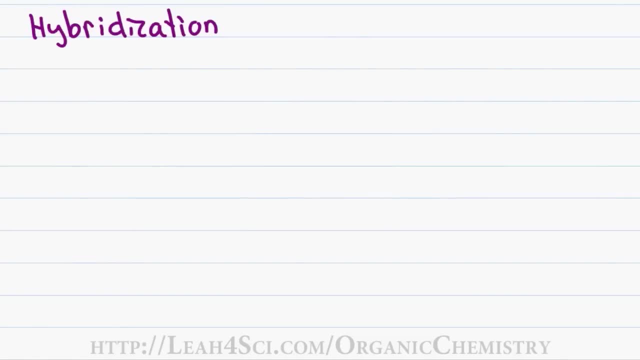 is taking orbitals that want to bond, orbitals that are not capable of bonding, and combining them into some hybrid that is able to create a bond with another atom. Let's look at carbon to understand this in more detail. The electron configuration for carbon is 1s2, 2s2, 2p2,. 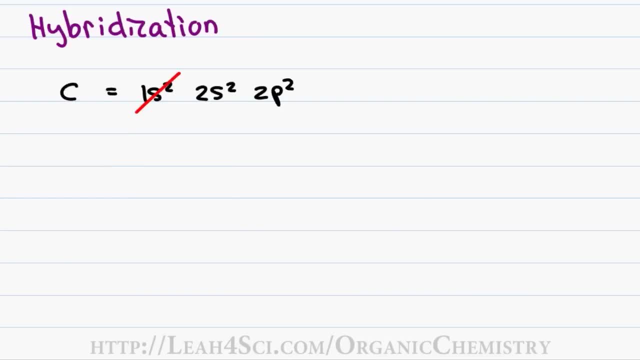 1s2 is the kernel or the internal shell, which we don't look at. It's only the valence shell that participates in bonding and in this case we have two electrons in the 2s orbital and two electrons in the 2p orbital, If we draw this out in terms of where the electrons are. 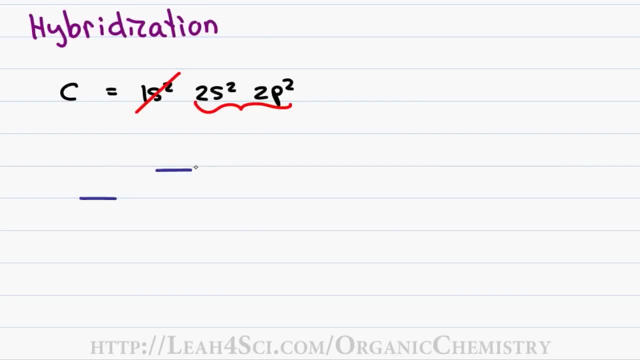 located and their energy. we have 1s orbital and three p orbitals. The s orbital is full with two electrons. The p orbital has just two electrons and one p orbital. The p orbital has two electrons between the three sub orbitals In order to create a covalent bond. another 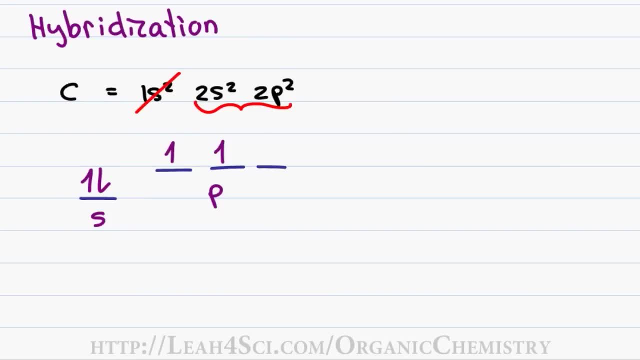 atom will have to take one of its electrons and combine it with a free or an available electron. If we look at carbon the way it is, we can have an electron bind with this p electron, another electron bind here, giving me a total of two bonds. But we know that. 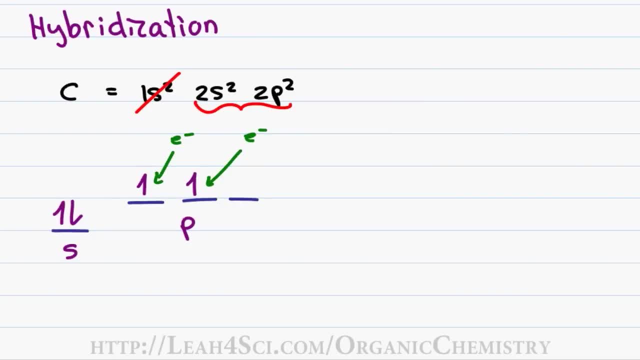 carbon, as the core atom in organic chemistry, is capable of forming four bonds. but how is that possible? To form the four bonds, we have to somehow combine the orbitals and the electrons from s and p and create a hybrid as follows: Bonding requires energy, and that slight bit of energy. 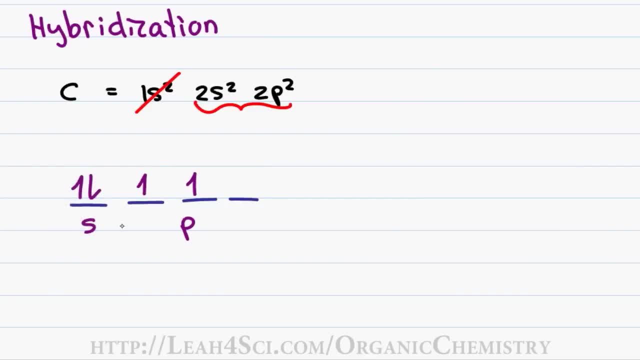 will take the low energy s orbital and raise it up to become equivalent with the p orbital. The electrons are now considered to be degenerate meaning of the same energy, and if we have degenerate electrons they will prefer to be spread out over the individual orbitals. 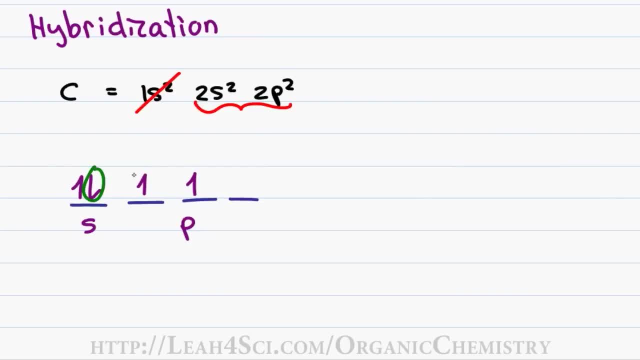 instead of being doubled up if there's still an empty orbital available. As I explained in my orbital video, the idea is: would you share a room with your sister if you had an empty room in the house? No, I personally would want to have my own room if I didn't. 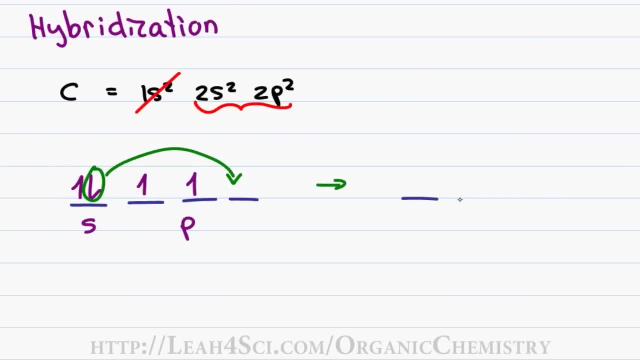 have to share with the sibling. What we have now is some mix of four sub orbitals containing a total of four equivalent electrons. To create this combination, we have to combine 1s and three p orbitals. One plus one equals zero. The other two have to be divided by three. 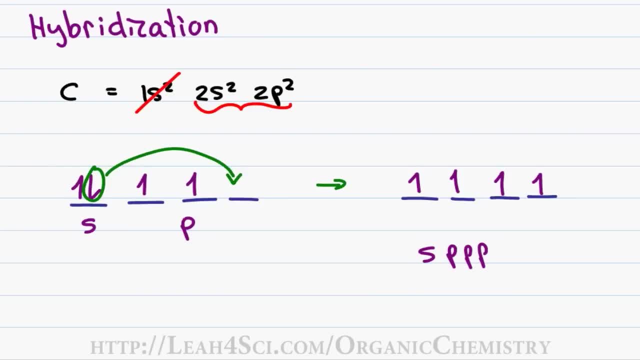 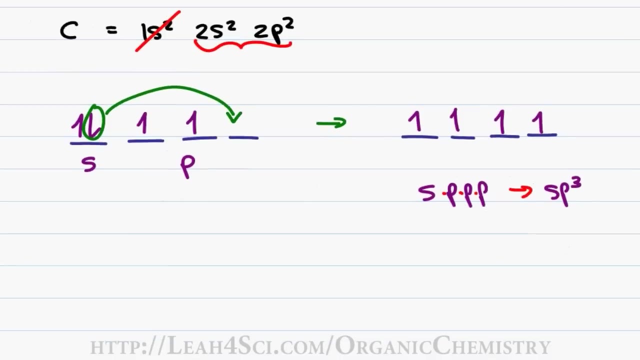 orbitals, and the designation for this would be S times P, times P times P. In math, when you have something times itself, it becomes squared, times itself again becomes cubed, and so the hybrid orbital is sp cubed, or simply sp3.. An example of this would be the molecule: 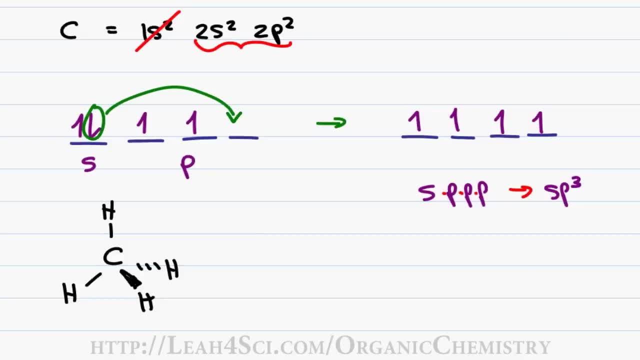 methane, We have carbon single bound to 4 hydrogen atoms. When carbon is in sp3 hybridization, we have 4 equivalent sp3 hybrid orbitals and each hydrogen atom is capable of binding to one of them. If you looked at methane and had to figure out the hybridization, here's: 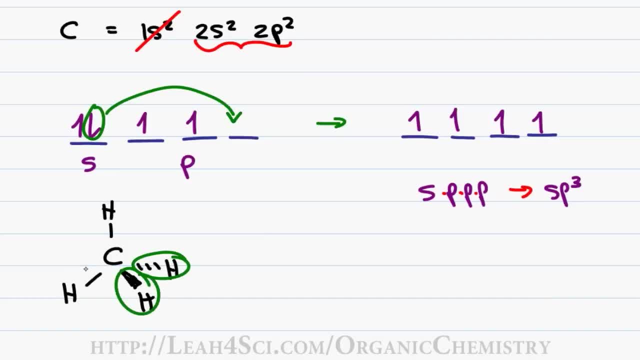 the trick: Count your bonds or groups. in this case, we have 1,, 2,, 3,, 4, draw 4 lines and then start counting from S to P, knowing that there's only 1S, 3P, anything beyond. 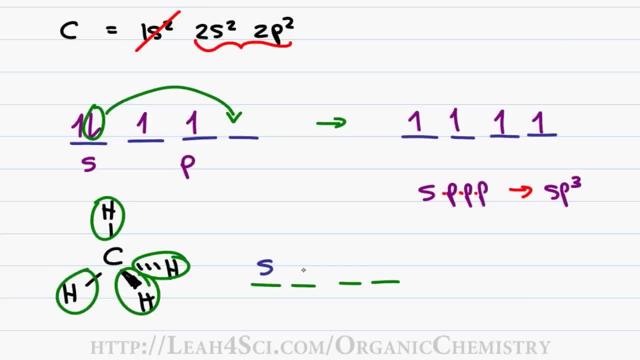 that becomes D. If we fill it in, we have S, and then we followed a P, P and P and then P, and that gives me sp3.. In order for four groups to be equidistant from each other, we get a bond angle, or theta, of 109.5 degrees. This is a number that you do have to memorize. 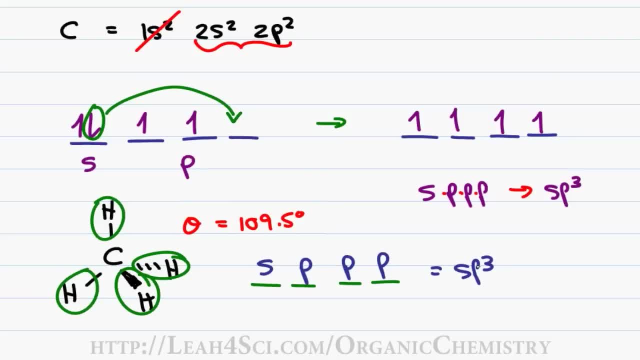 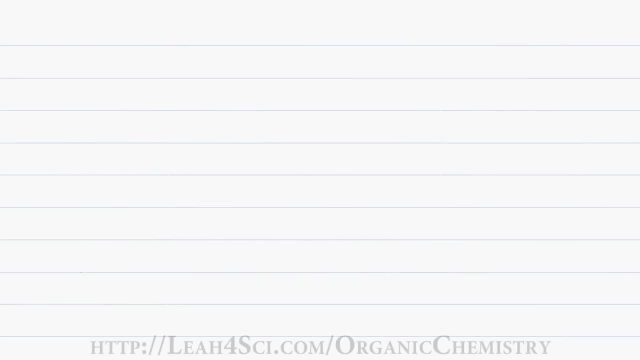 sp3 hybridization is typically 109.5.. Sometimes the number will be slightly greater or slightly less if there's difference in polarity between the atoms that bind to that central atom. but that's the number to memorize. b atoms that are not carbon, that will also undergo hybridization, but it's a little bit harder. 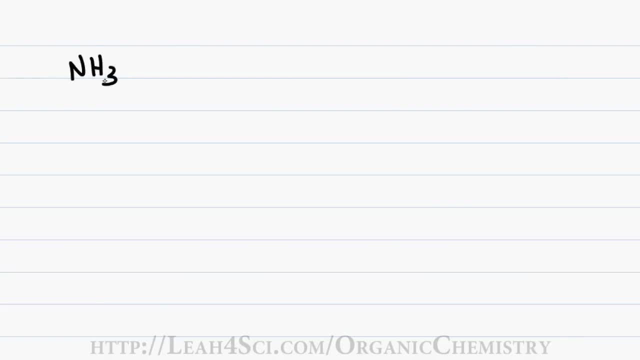 to see. For example, if we look at nitrogen in NH3, nitrogen is bound to three hydrogen atoms. It also has two valence electrons. If we look at the electron configuration for nitrogen, we have 1s2, 2s2, 2p3.. 1s2 is the kernel. we get rid of it. 2s2 and 2p3 are 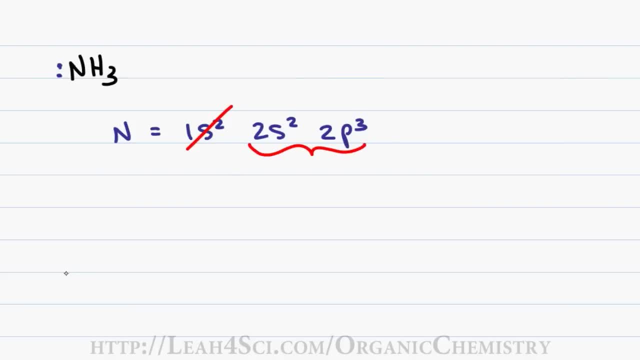 the valence electrons. We have the 2s with two electrons and 2p with three electrons. As it is, it looks like the nitrogen is capable of binding to the hydrogens without any change or hybridization. But when you have lone pairs of electrons in a molecule, almost think of. 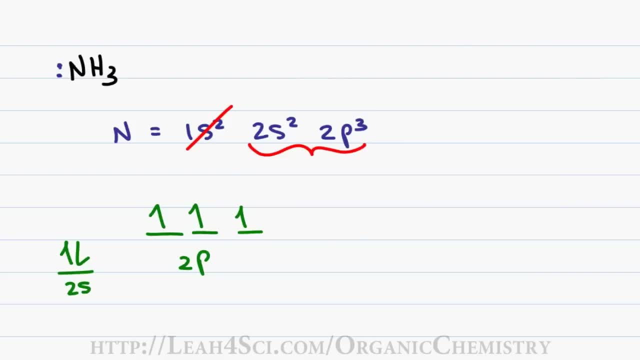 it, as the electron is bound to the other electron and therefore it has to be at the same or very similar energy level. So in this case we'll still elevate the s to the level of p and have the combined hybrid orbital of sp3.. The way you want to envision this is as follows. Remember, for carbon, we 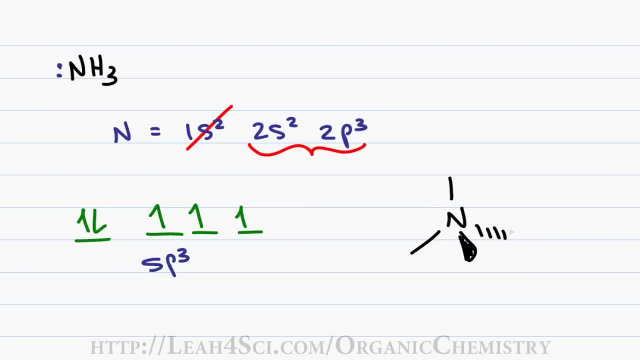 drew our shape like this, showing four equal units with a tetrahedral geometry. We'll bind our three hydrogens because we know that's there For the fourth one, instead of putting a lone pair. just imagine as if the electron is bound to the other electron. It's not? 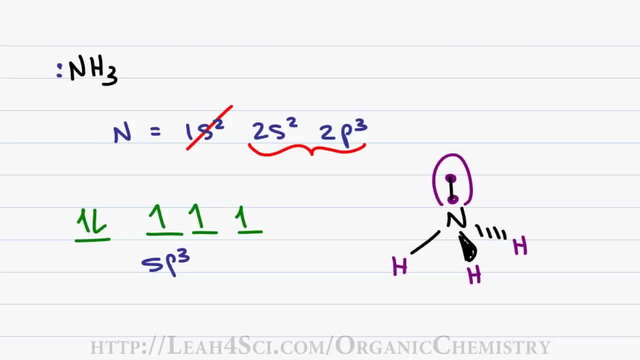 NBA. not really, They're in their together, but this is how you can understand that, even though we have only three bonds, it's still a tetrahedral electronic configuration. The reason I stress electronic is there are two ways to look at this shape For the electronic. 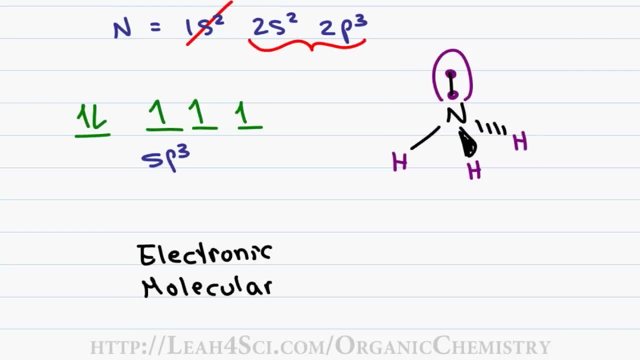 geometry, we're looking at where the electrons are located. we're not looking at the atoms that they're bound to, So, for example, nitrogen bound to hydrogen. we're only looking at the bond, which is an electron on an electron. Just like with the lone pair, we have the 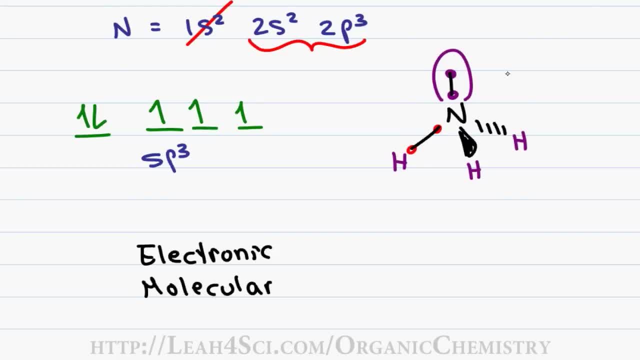 electron and electron. The electronic geometry which comes from the sp3 hybridization has four different groups, giving me a tetrahedron as the noun or tetrahedral as the verb. same thing, But if we look at just the molecule, meaning only the visible atoms, we have nitrogen. 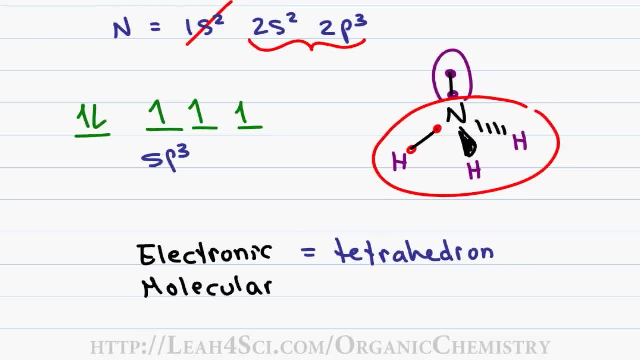 bound in a weird pyramid to the three hydrogen atoms, ignoring the effect of the electrons. the molecular geometry is actually trigonal-pyramidal. The trigonal comes from the three atoms, which is a triangle shape, but the pyramid tells us that it's bent slightly downward from the 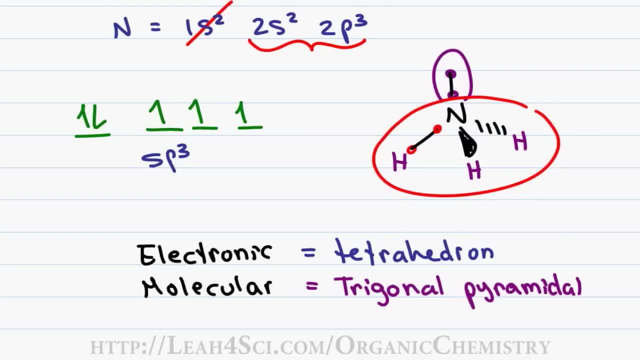 nitrogen and forms a pyramid rather than being flat. This is why you should know both the electronic and the molecular, Even though we have the triangle shape from the hydrogens, that lone pair of electrons being more negative compared to the atoms that are sharing is. 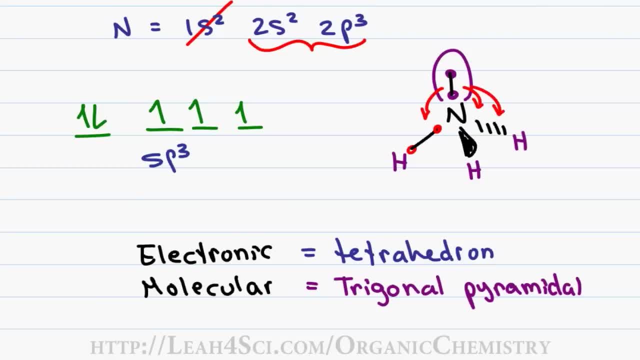 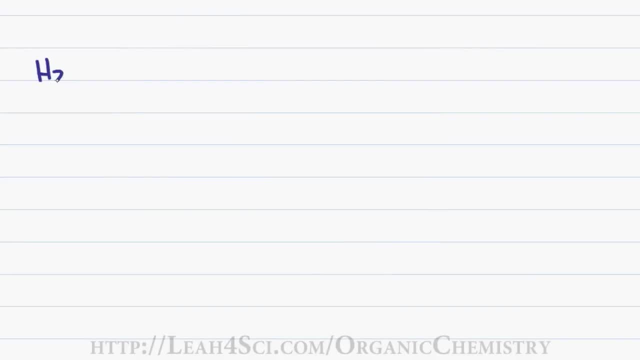 going to repel the bonds downward, forcefully Infusing them into a pyramid, rather than allowing them to be flat, as we'll see later with sp2 hybridization. Let's look at one more example of an sp3 atom. This time we look at water, where oxygen is. 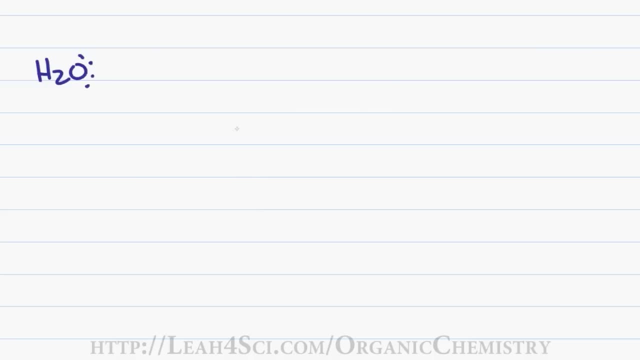 bound to two hydrogen atoms, but it also has two lone pairs. We'll draw the oxygen in a tetrahedral shape, given that it's sp3 and has four equal groups surrounding it. two of the groups will get a hydrogen atom where we have the bonds, and two of the groups will 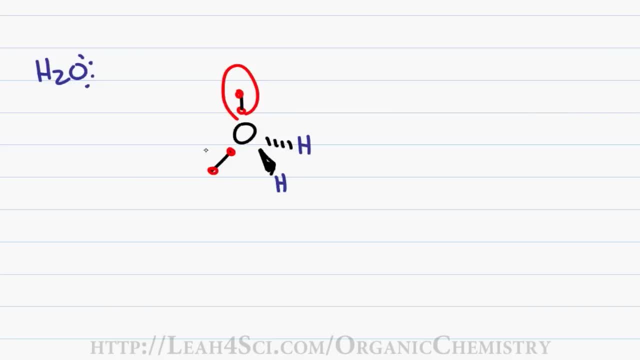 get an electron where they communicate as one, get an electron bound to an electron as our way of understanding how it's tetrahedral. Notice that even though we have the two atoms, we still have that overall sp3 hybridization. Since this is sp3, the electronic geometry is still tetrahedral, but the molecular geometry 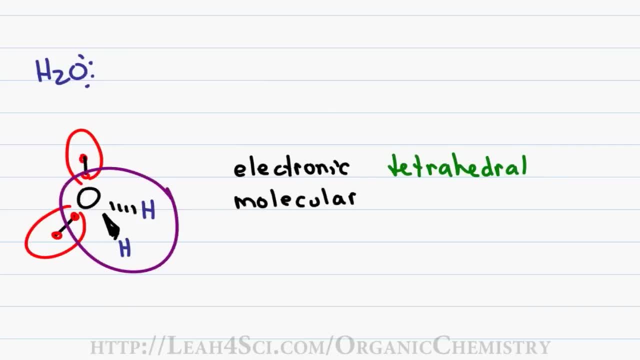 which only looks at the molecule visible and not the electron surrounding it, is going to be simply bent, because the oxygen has two hydrogen atoms and they're bent slightly towards each other. The bond angles are still approximately 109.5, but because the lone pairs are considered, 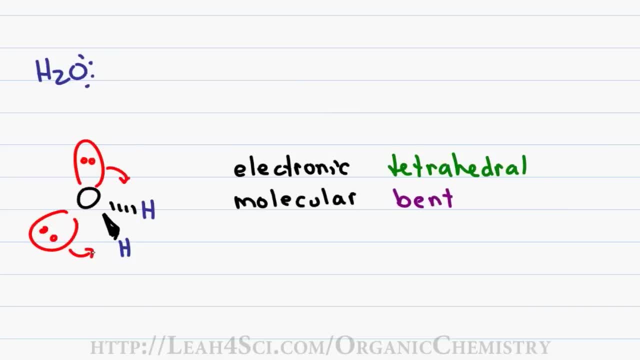 to be slightly more negative. they're going to push on the hydrogen atoms, forcing them closer together. If this was an exam and you didn't memorize the exact number, you can write slightly less than 109.5 for the angle between the hydrogen atoms and slightly greater than 109.5 for. 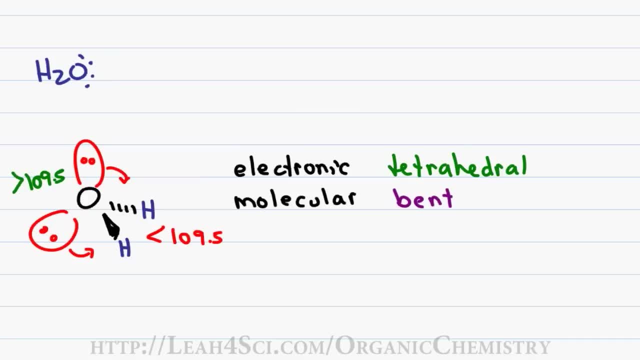 the electron. I think the angle is somewhere near 105, but unless you're told to memorize it, don't worry about it. But be sure to join me in the next video where I take you through sp2 and sp hybridization and then show you a fun trick for how to quickly recognize the hybridization on wacky molecules. 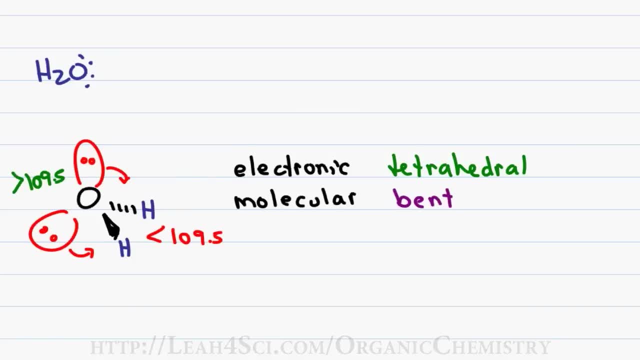 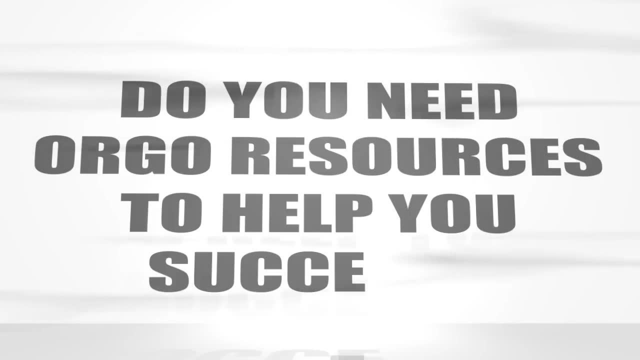 including drugs that professors love to put on exams. Are you struggling with organic chemistry? Are you looking for research? Are you looking for resources and information to guide you through the course and help you succeed? If so, then I have a deal for you.